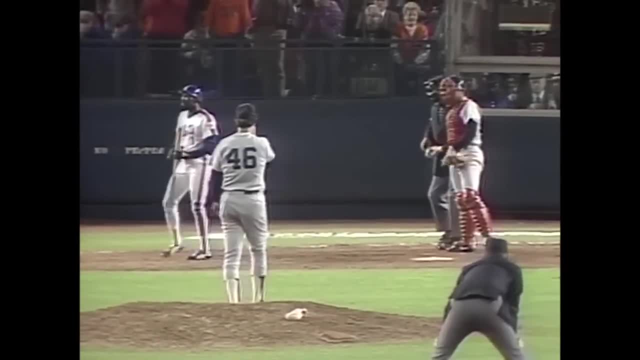 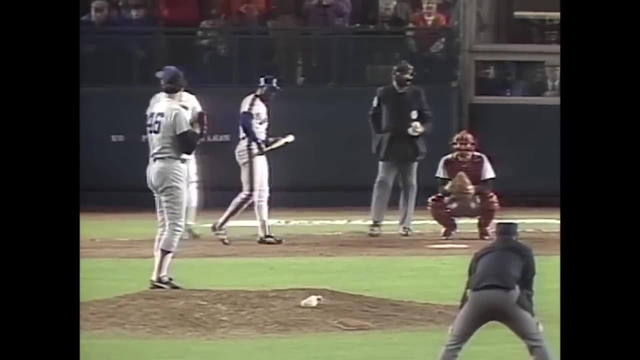 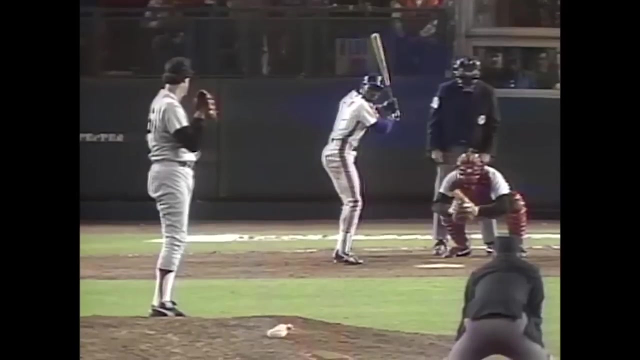 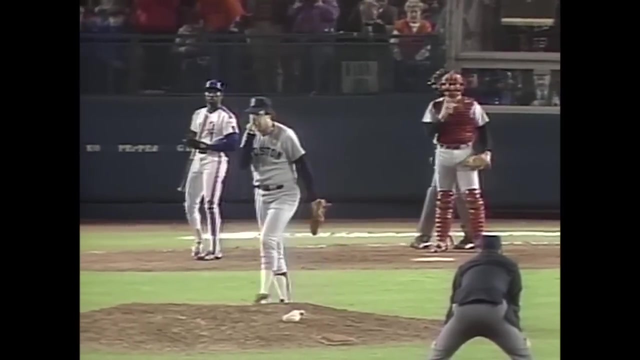 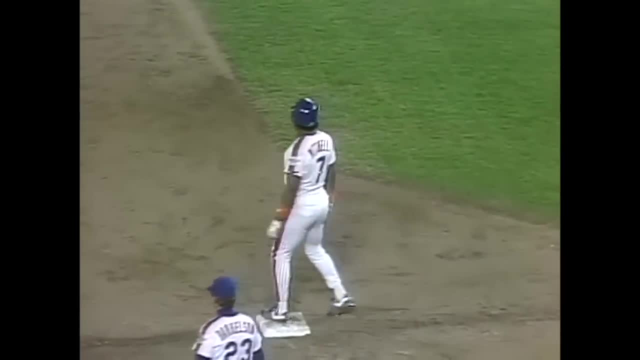 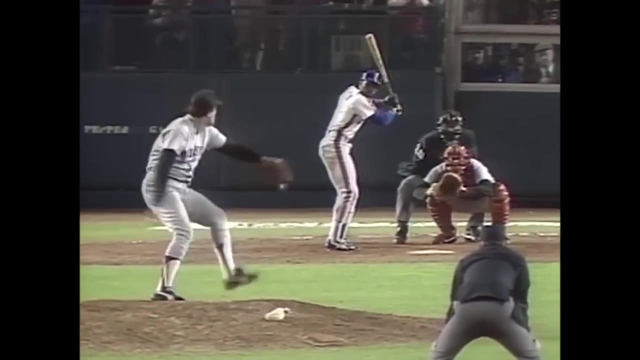 Five-four Red Sox: Ray Knight at first, Kevin Mitchell at third. Right at the end of the line, We're going to have two more two and two to Mookie Wilson and it's going to go to the backstop. here comes Mitchell to. 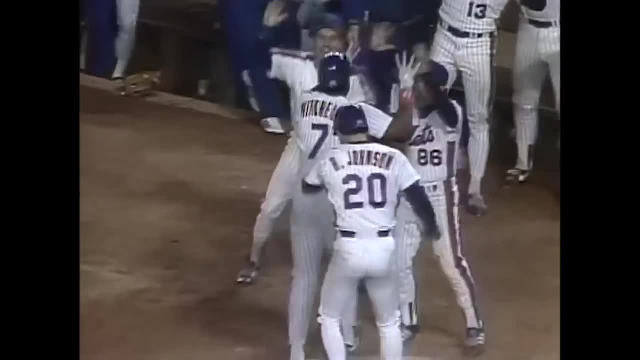 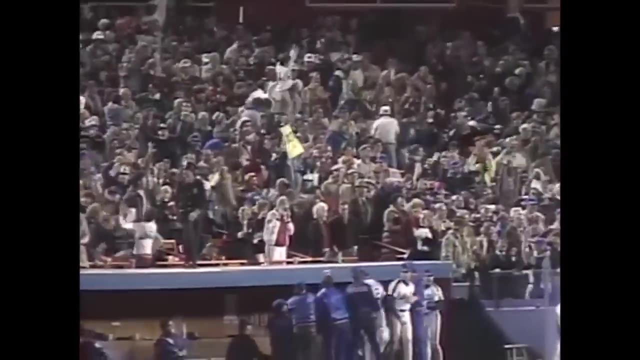 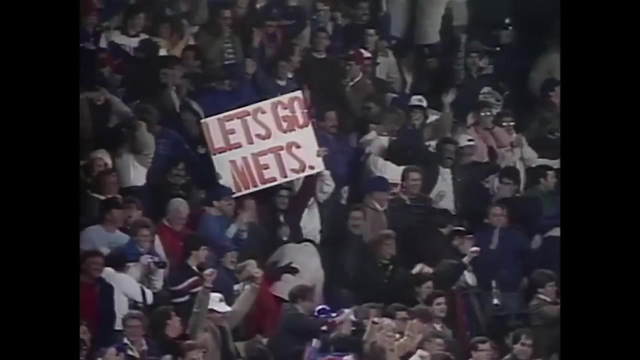 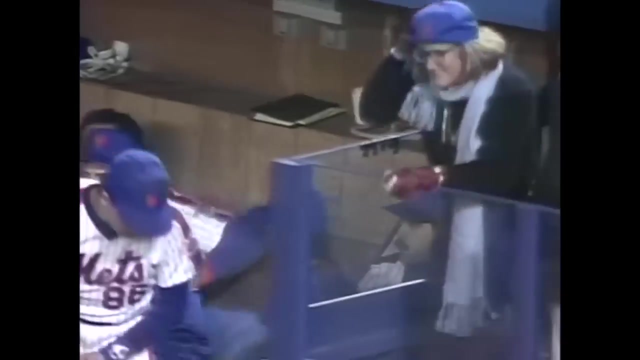 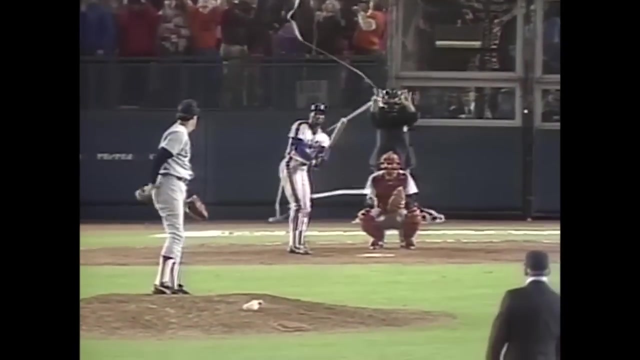 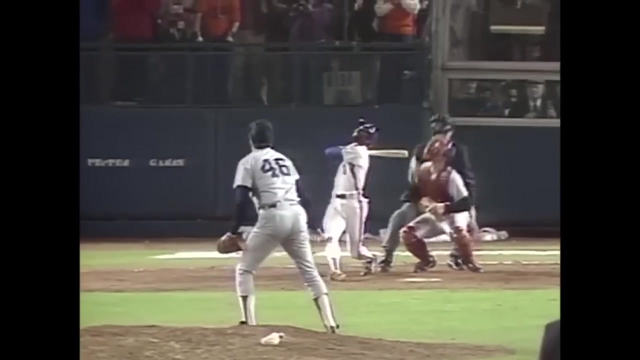 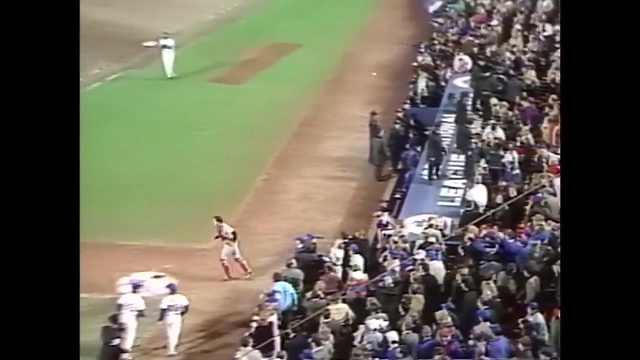 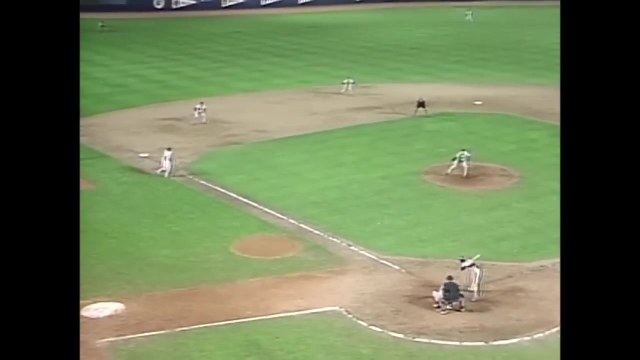 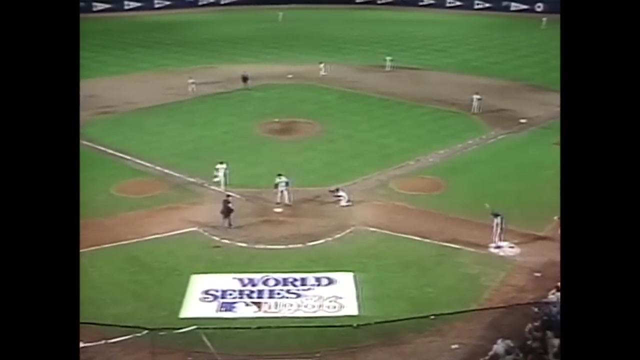 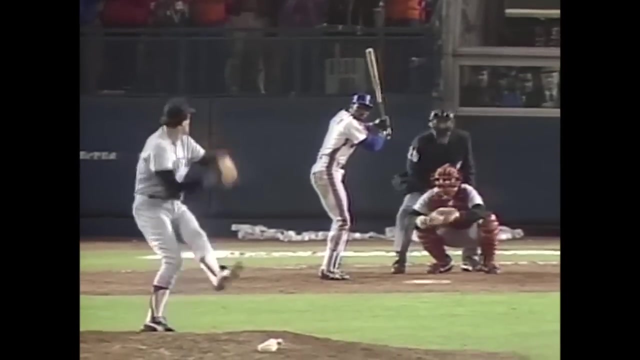 score the tying run and Ray Knight is at second base. three and two to Mookie Wilson and he pops it in the air foul off to the right, getting and coming over. he will not have a play. five, five and a delirious 10th inning line drive foul and 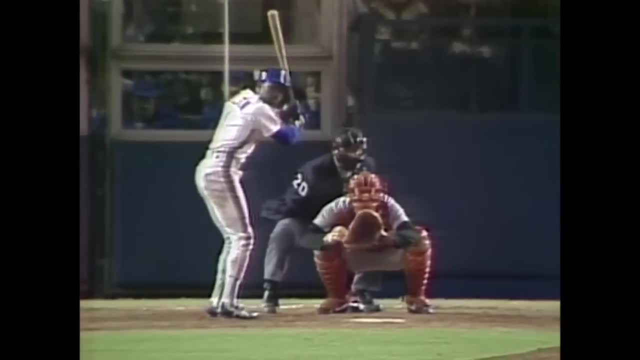 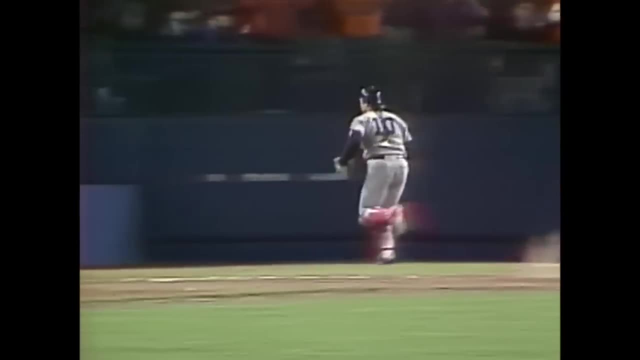 Marnie Barrett was out of position because they had night really picked up and Stanley didn't see him. there it is again, you see, he just reaches for the ball, down goes Mookie. it kind of sailed inside. and here comes Barrett in the talk to Stanley because had 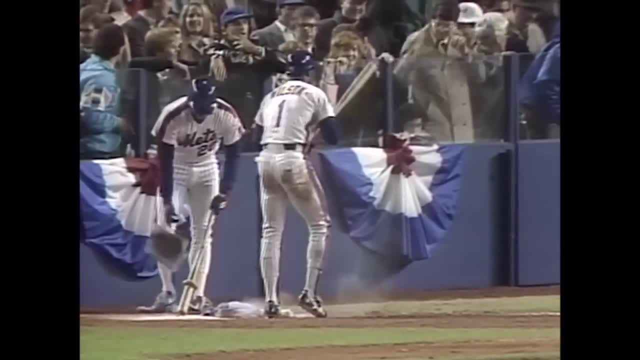 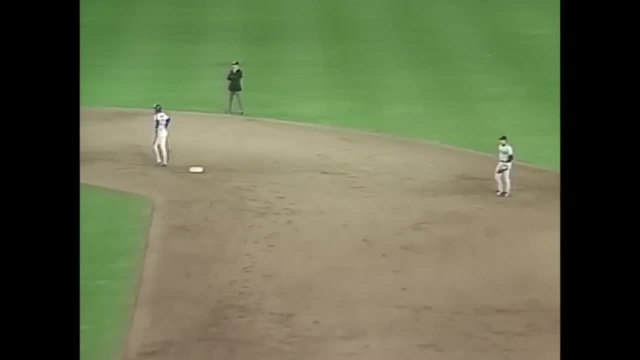 Mookie hit just a weak ground ball. Barrett was way out of position because they had a good chance to get night at second base. can you believe this ball game at Shea? oh brother. so the winning run is at second base, with two out, three and two to. 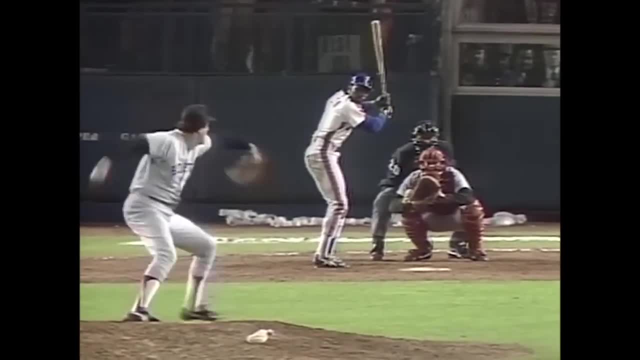 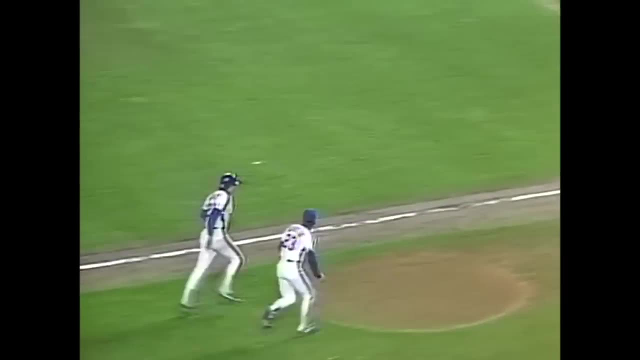 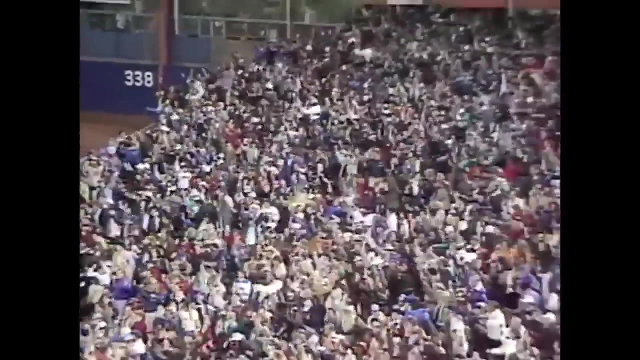 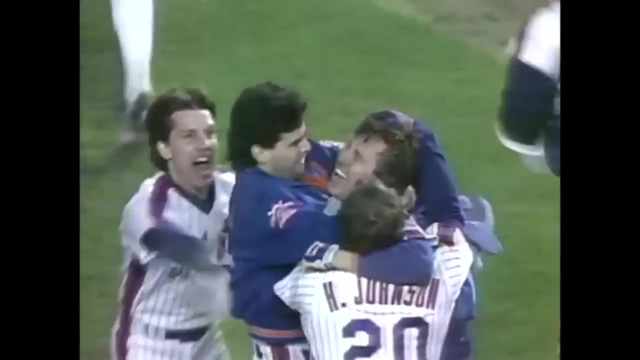 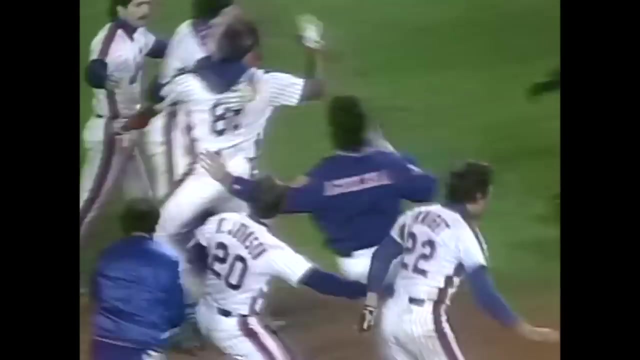 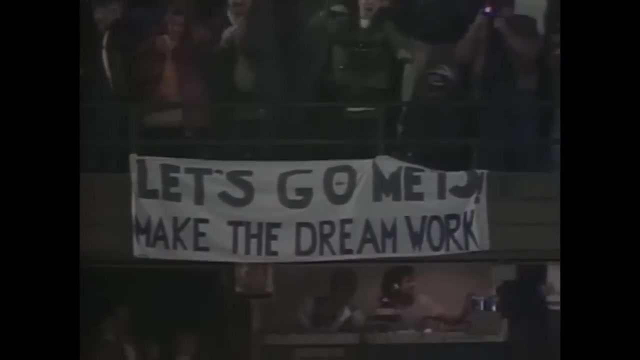 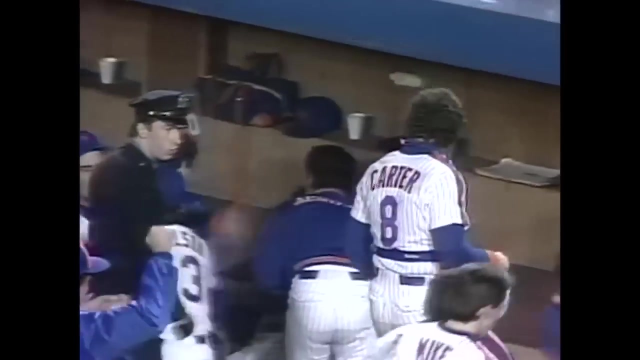 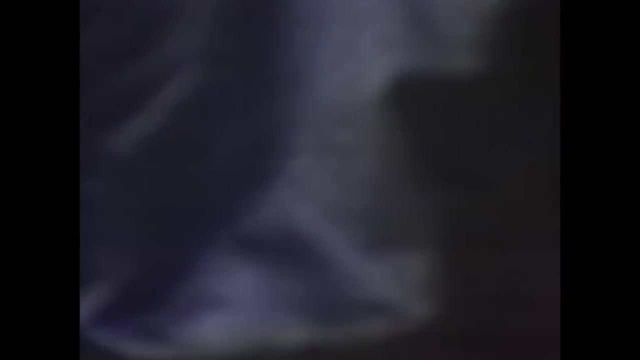 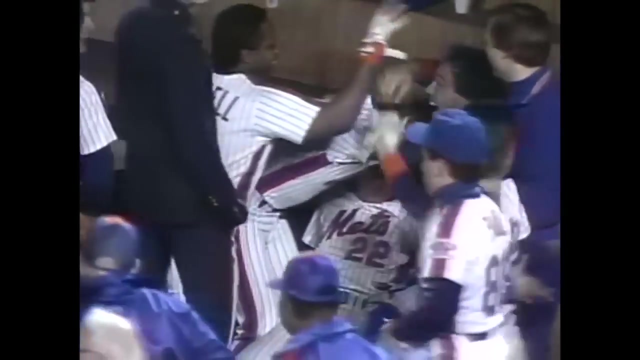 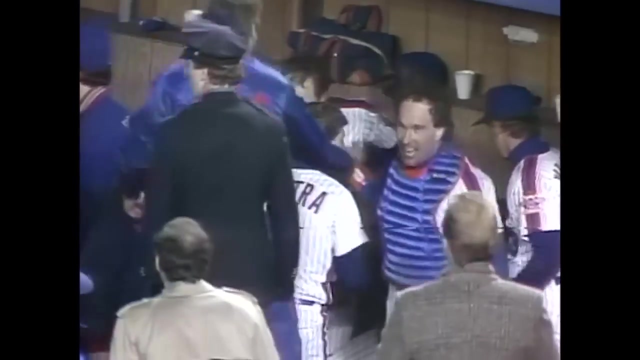 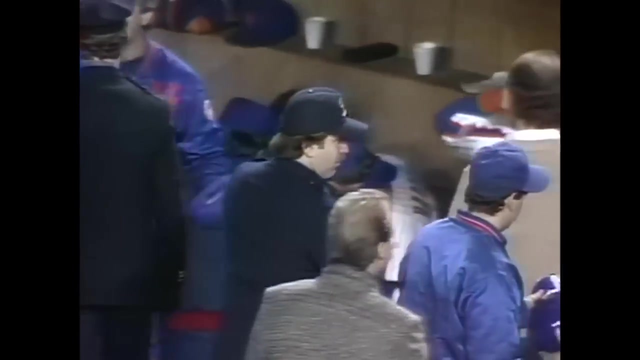 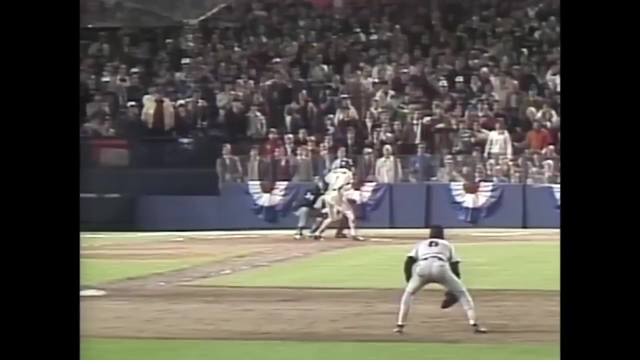 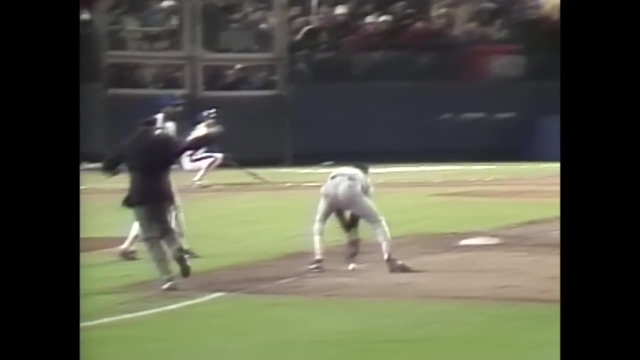 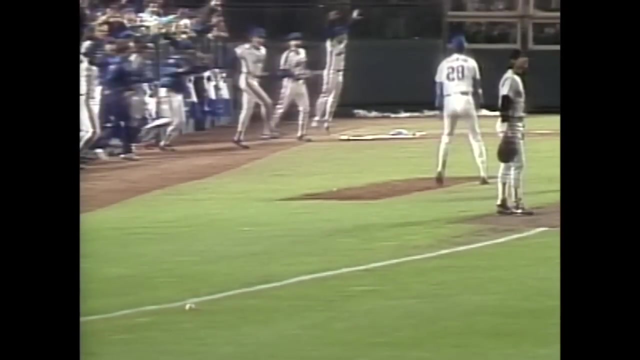 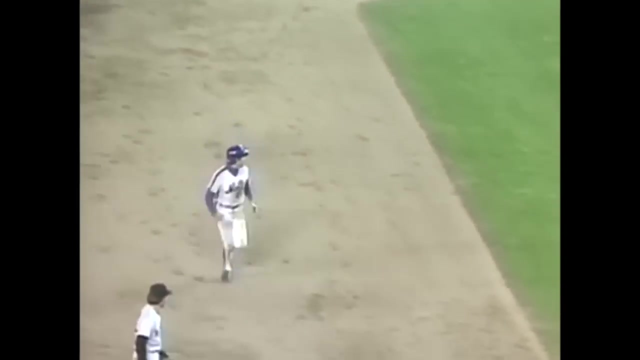 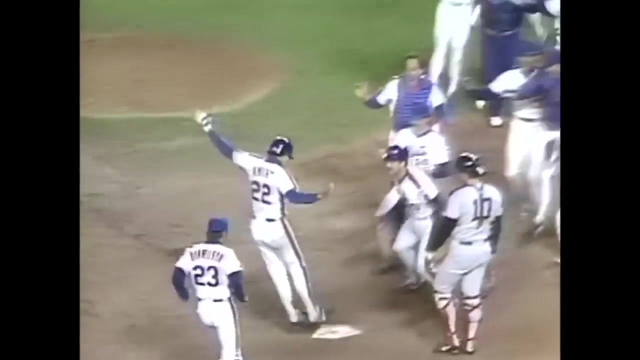 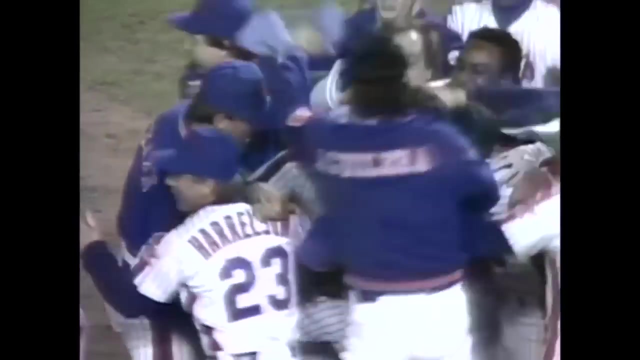 Mookie Wilson, little roller up along first behind the back, it gets through Buckner. here comes Knight and the Mets win it 3, 2, 1, 0, 6, 7, 6, 7, 8, 9, 10. Thank you, If one picture is worth a. 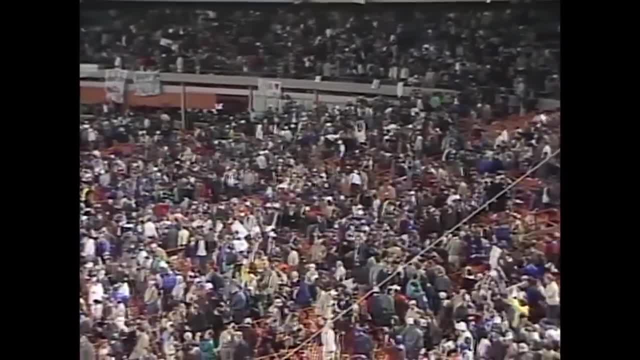 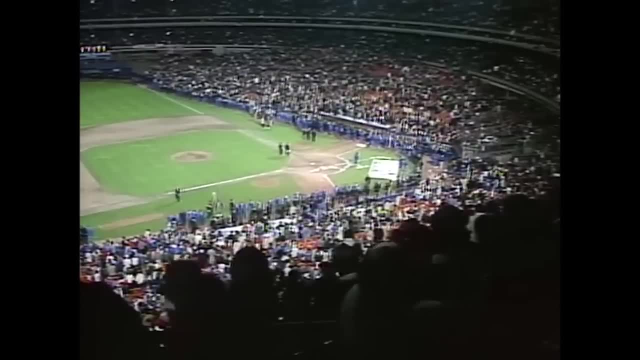 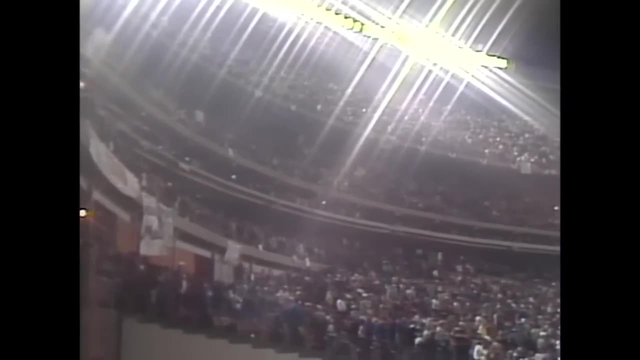 thousand words. you have seen about a million words, but more than that, You have seen an absolutely bizarre finish to game six of the 1986 World Series. The Mets are not only alive, they are well, and they will play the Red Sox in game seven. tomorrow.